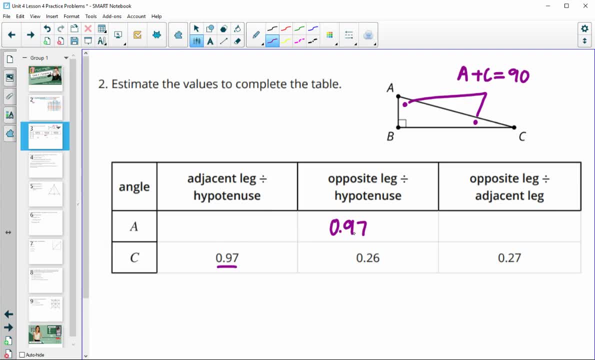 point or goes to the opposite. So adjacent over hypotenuse moves to opposite over hypotenuse, And opposite over hypotenuse moves to adjacent over hypotenuse. Then for this final category here you can take, this is opposite divided by adjacent. 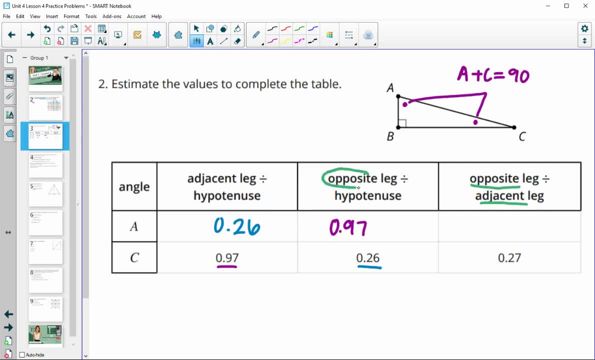 So opposite divided by adjacent. So we'll take the column with the opposite, which is 0.97.. And we'll divide that by the column with the adjacent, which is 0.26.. And that will give us about 0.7,- oh sorry, 3.73 for this one. 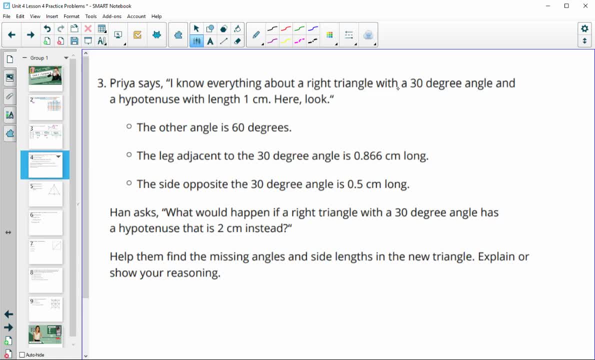 Number three, Priya says I know everything about a right triangle that has a 30 degree angle and a hypotenuse of one centimeter. Here look. So let's kind of fill out what she tells us as we go. So she said: if it gives her. 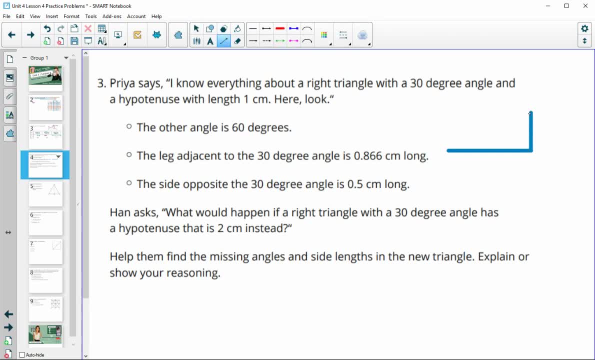 a 30 degree angle and then a hypotenuse of one. she'll know everything else. So if she was given this is 30 degrees, it's a right triangle, and then the hypotenuse was one centimeter, she says she knows everything else, So she knows that this angle is going to be 60,. 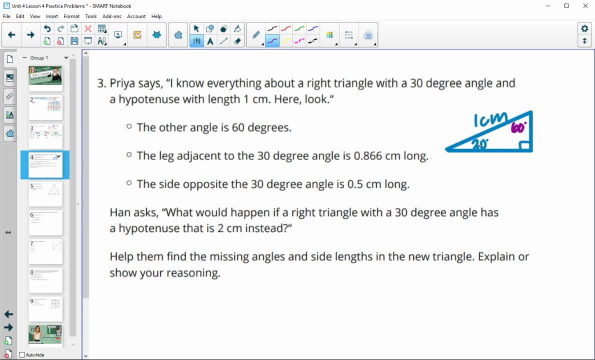 that the leg adjacent to the 30,- so next to the 30, is going to be 0.8.. So that's going to be 0.866 centimeters long, and that the leg across from the 30 degree angle is going to be 0.5 centimeters. So then Han asks: I wonder what would happen if the hypotenuse was. 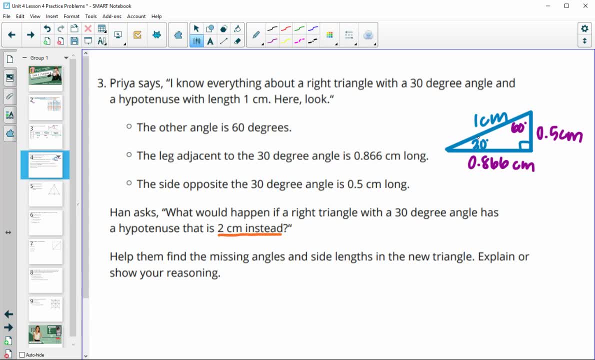 actually two centimeters instead. So we know that the triangles are going to be similar because they have all the angles the same. So if this one is now two centimeters long, we would just need to figure out a scale factor. So this is going to be twice as big as one centimeter. So the scale. 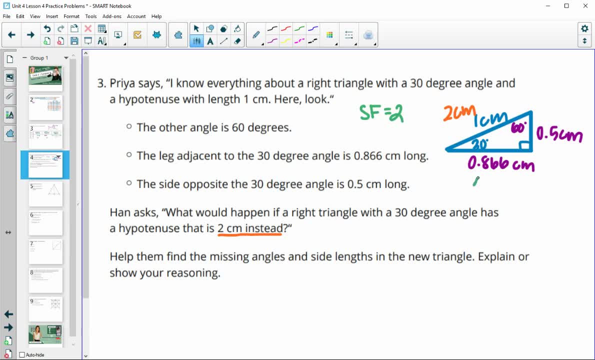 factor is equal to two, So the other side lengths are just going to be twice as long. So we would just multiply these together, or multiply these by two, and that would get us the new side lengths. So this new adjacent side would be 1.73 centimeters. 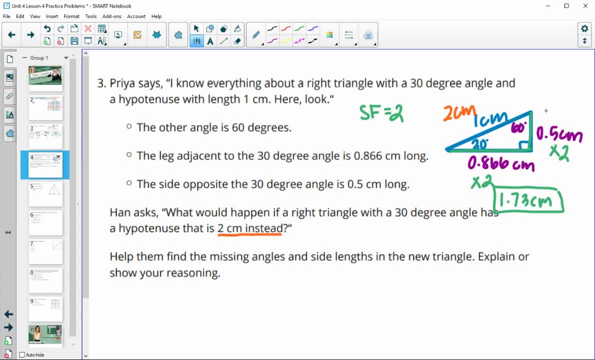 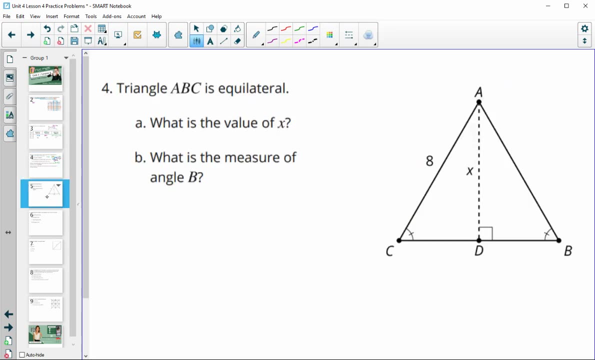 And 0.5 times two would make this new opposite side be one centimeter. if the hypotenuse was moved to two centimeters and the angles would stay the same. Number four: this triangle that they give us is equilateral. Find the value of X. So we know that. 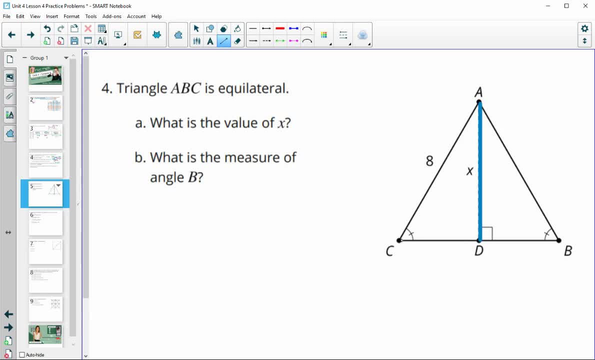 X is this altitude, and we know that the altitude is this short leg times the square root of three, when we're in X. So we know that X is this short leg times the square root of three when we're in X, And we know that this length here is half of the whole side. So this is four. So you can think of it. 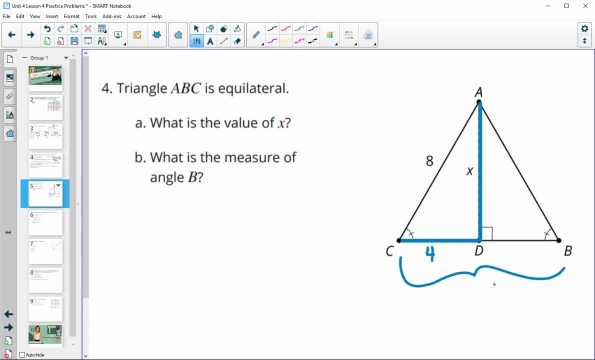 as half the hypotenuse. You can also remember that it's half of this length here, which is also eight. So this is four, and then this altitude will just be that shorter leg times the square root of three. So X is going to be four, square root three. And then what's the measure of angle B? So remember. 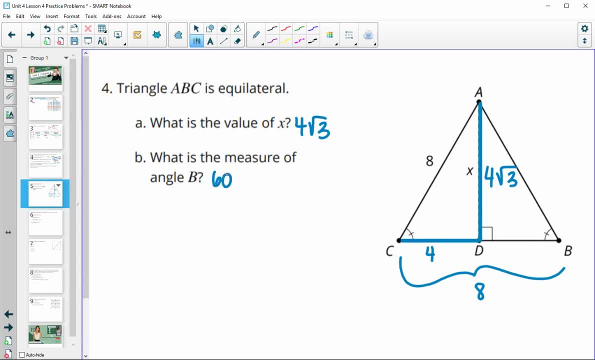 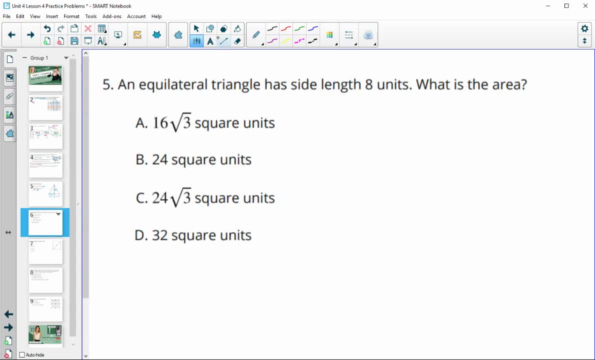 this was an equilateral triangle, which is also equiangular, So we know that that angle B will be 60 degrees. Number five: an equilateral triangle has a side length of eight. What's the area? So we could draw an equilateral triangle here. We know that the side length is eight. We need the altitude. 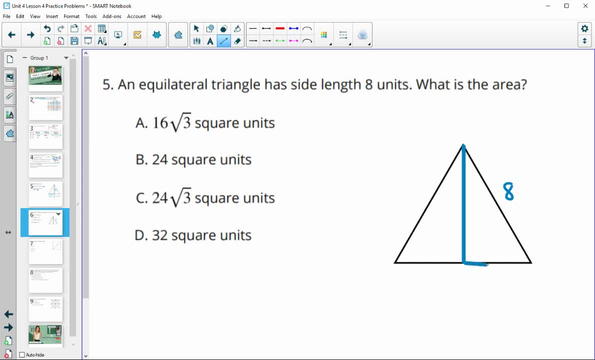 to find the area And we know the altitude is the square root of three times bigger than this segment. So we know this segment here is four, since it's half of the eight down here or half of the hypotenuse. And then we know this altitude is just going to be that leg times the 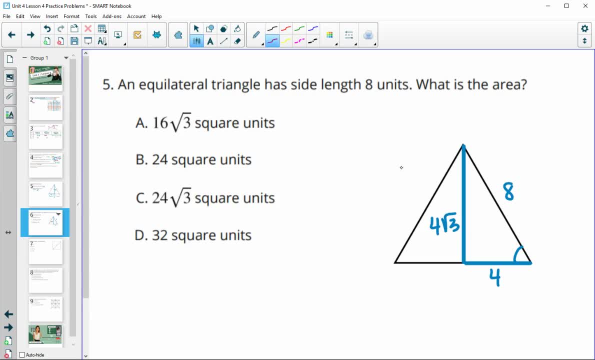 square root of three, So four, square root three. So then when we go to find the area, we'll do the base, which is this whole length here, which is eight, since all the sides are the same length times the height, which is that altitude. 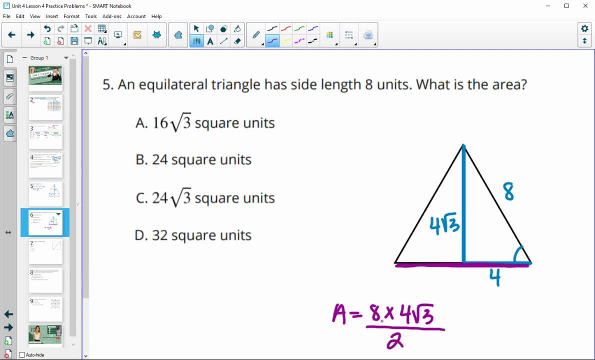 or square root three divided by two. That's the area formula for a triangle: base times height divided by two. So on the top here we get 32 square root three divided by two. So we'll do the 32 divided by two and get 16 square root three And then, since it's area, we'll also have square units. 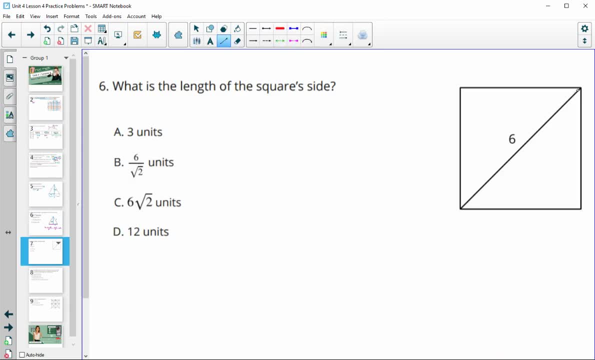 Number six: what is the length of the square's side? So we know that a square creates a 45-45-90 triangle, And we know that in a 45-45-90 triangle the hypotenuse and the leg are a square root of two factor away from each other. So if we 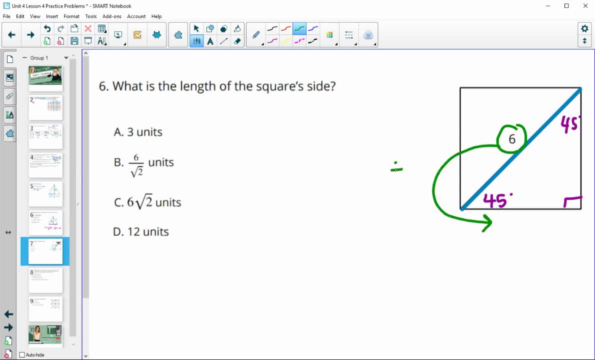 have the hypotenuse. we divide to get the leg, remembering that the leg is shorter than the hypotenuse. So we'll divide by square root of two. So this leg is going to be six divided by square root two. And that is answer choice B. 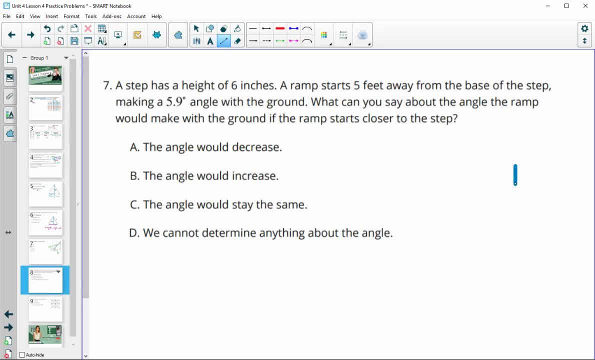 Number seven. a step has a height of six inches, And then there's a ramp that is five feet away And it makes a 5.9-degree angle with the ground. So let's just fill this out. So we've got this at six inches. 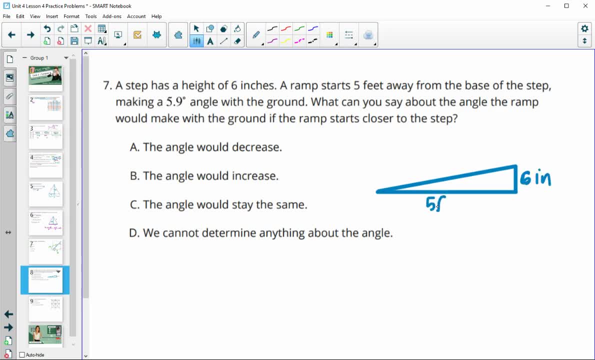 and then the ramp is five feet away and then we know that this angle here is 5.9 degrees. What can you say about the angle of the ramp if the ramp starts closer to the step? So if we moved this ramp closer to the step, so we ended up more with this triangle here, so we could say that this? 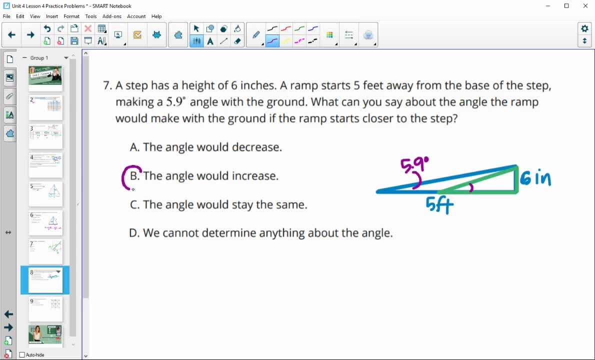 angle right here is actually getting bigger. It's going to increase. That's because we can see that this angle up here is the green angle up here is smaller than this blue angle because it's contained inside. We know this stayed 90, so if this one is getting smaller, this one has to be. 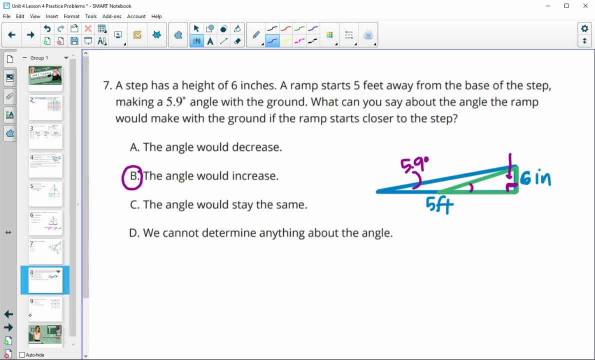 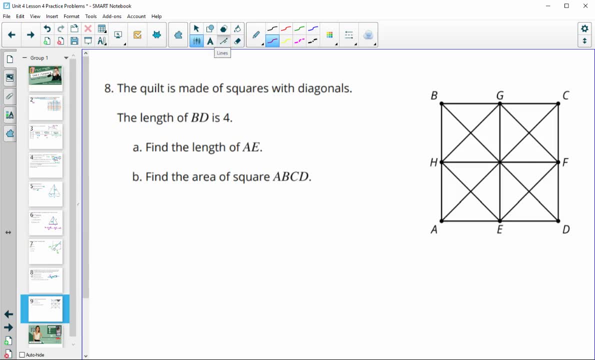 getting bigger, since we know they always total 180.. Number eight: we have this quilt design that's made with square diagonals. The length of BD, this segment here, is four, and then let's find the length of AE. So AE is this piece. 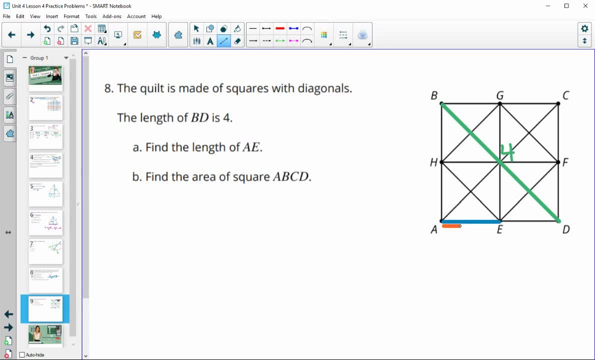 So first we can go ahead and find the length of AD, and then we know AE will be half of that, and so we see this 45, 45, 90 triangle being created here, since it's half of that square. So we know that this is going to be half of that square, and then we know that this is going to be.